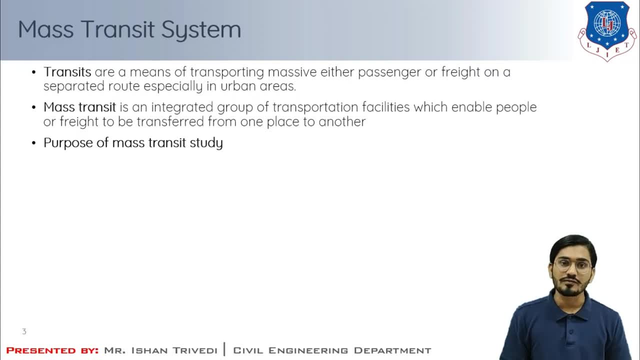 To study the operations, problems and the location of stops- And that's why we require mass transit study- To establish the extent of uses and determine the vehicle types and various routes, Then to obtain the characteristics of mass transit riders. Then to plan, design and operate mass transit services. 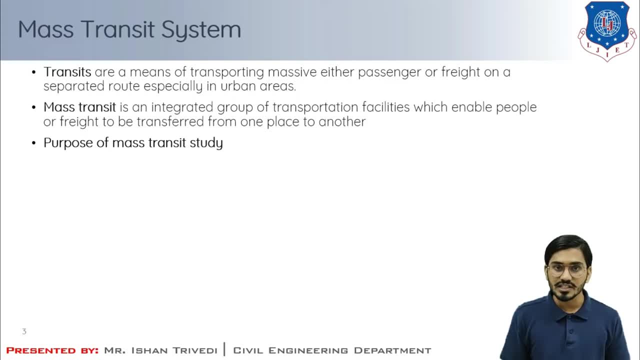 Then scheduling of these mass transit services. Then to conduct an economic analysis of public transport And the various operations which has been carried out for this public transportation and their improvements. Now there are the classification of mass transit system On the basis of technology, or you can say transit technology. 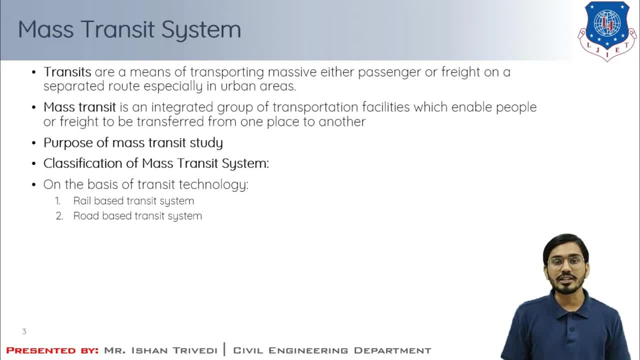 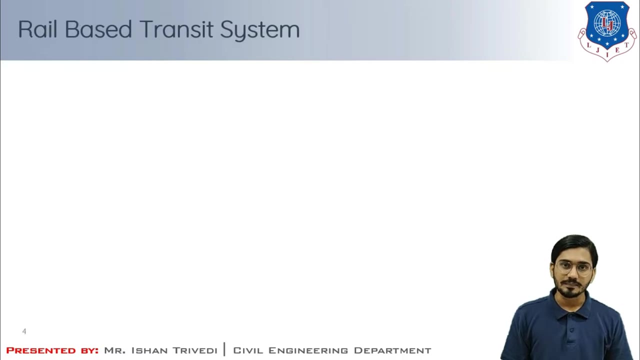 Mass transit systems are classified in two parts, That is, rail based transit system and the road based transit system. In this session I am going to cover rail based transit system. So now let us start with the rail based transit system. It mainly classifies in four categories. 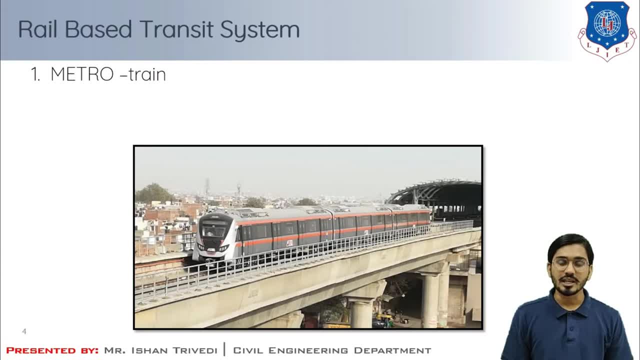 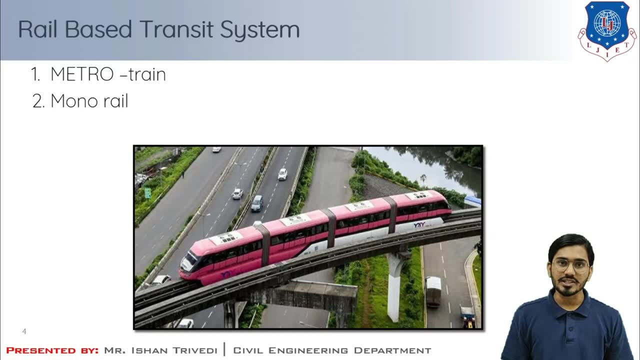 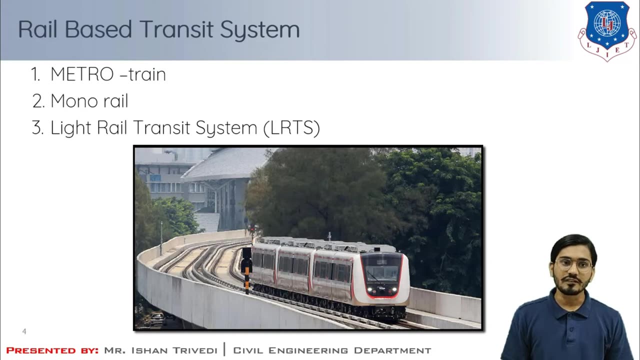 First is metro train. This is the image of Ahmedabad metro. Second is mono rail. In Mumbai the transportation is been done by this mono rail, Then light rail transit system. It is one of the updation of metro train Where two to three 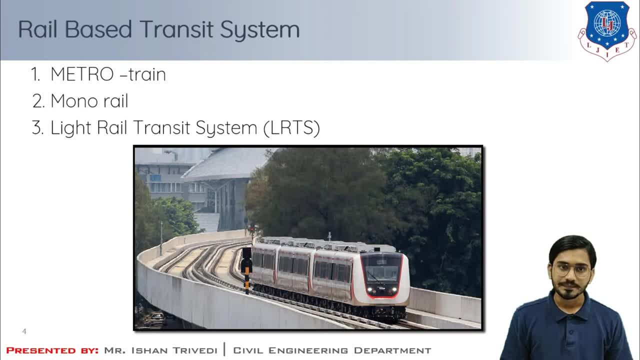 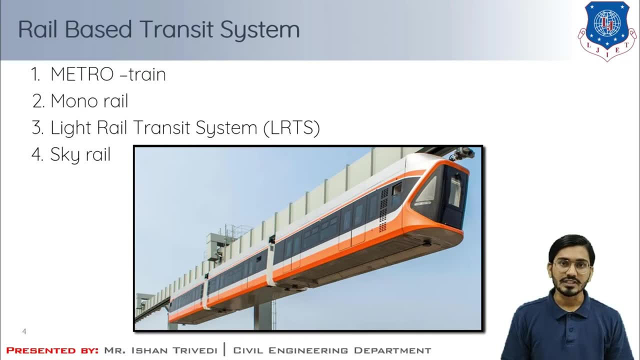 Or you can say, articulated service has been provided. Next is sky rail. This image is from China. In China, many of the cities are upgraded with the sky rail. You can have this case study and understand how they have come up with this new phenomenon. 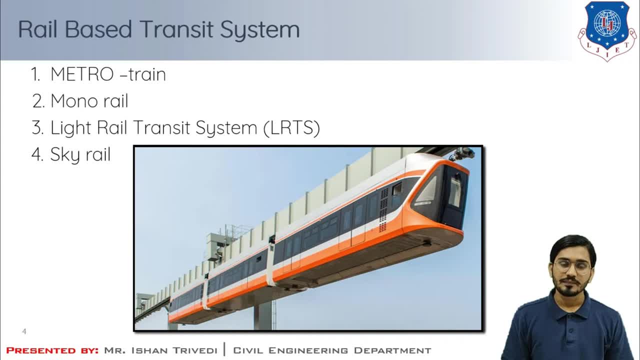 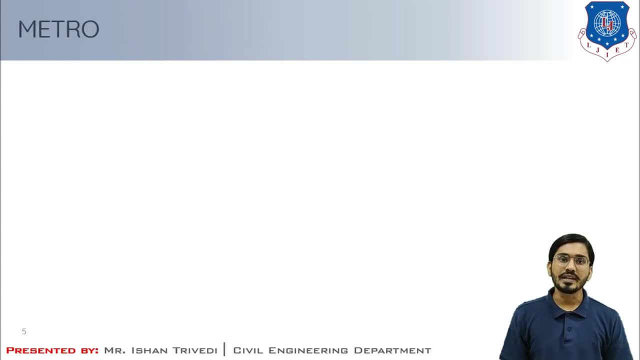 I will discuss here brief introduction of these four transit system. So first let us start with the metro trains, Or you can say rapid rail transit, RRT. The first modern rapid transit in India was Calcutta metro And it was started in its operation in 1984.. 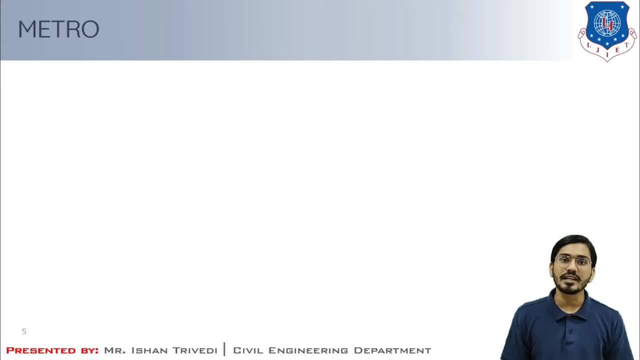 Then Delhi metro in New Delhi is the second conventional metro, which began in 2002.. Afterwards, the Bengaluru metro services were there And in many of the cities, like Ahmedabad and the other cities where the metro runs in a particular dedicated corridor, As well, as some of them are under the construction or some of them are under planning stages as well. 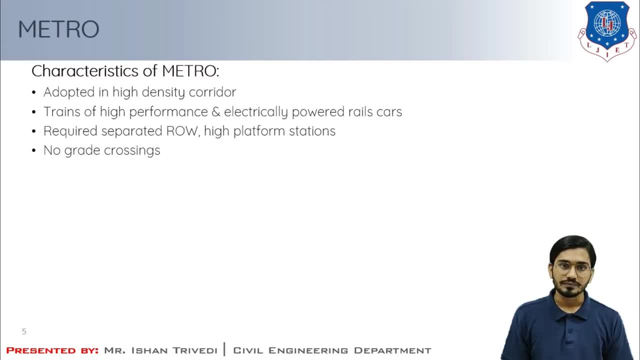 Now understand the characteristics of metro. Metro are usually adopted in high density corridor of densely urbanized area. It uses the train of high performance and electrically powered rail cars. Metros require fully separated right of way with manual, signal or automatic control. They require high platform, stations at elevation, or sometimes it is at grade or at subgrade. 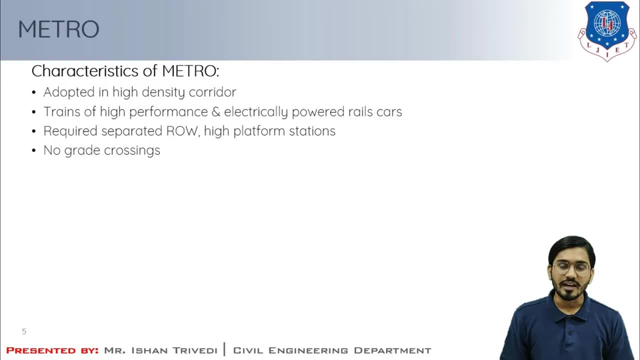 In this metro route there are no requirement of grade crossing. That means a dedicated railway track is there and road is crossing over it, Or you can say a signalized where a railway and a road crossing each other. So there is no requirement of any grade crossing. 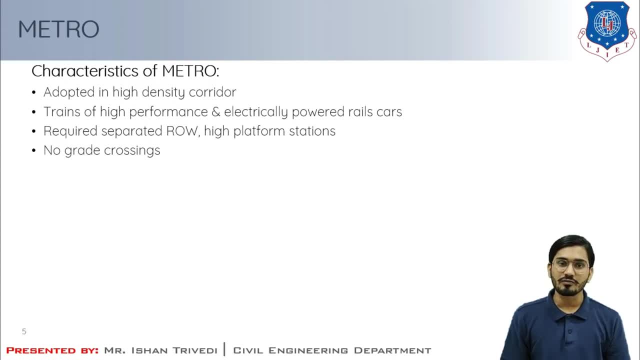 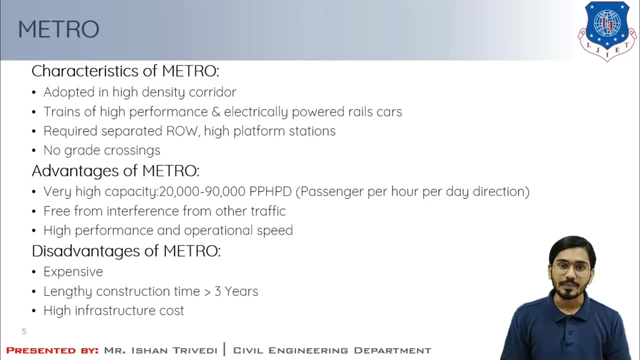 Then if I am talking about advantages and disadvantages of metro, These are: if I am talking about the advantages of metro, It has very high capacity of passengers. It is almost around 20000 to 90000. pphpd means passenger per hour per day direction. 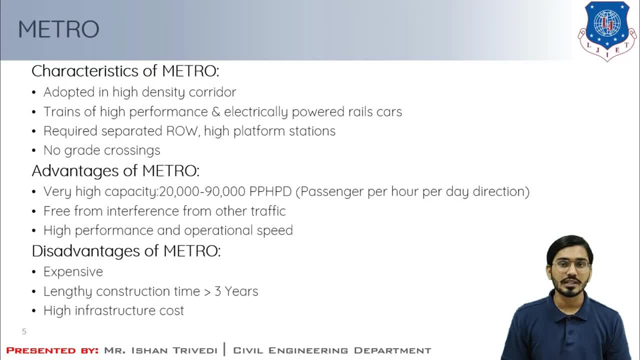 It is free from the interference of other traffic And that's why the travel time can be minimized. Then it has very high much performance and operational speed. If I am talking about the disadvantages, It is most expensive option There may be. require high infrastructure cost which elaborate the stations as well. 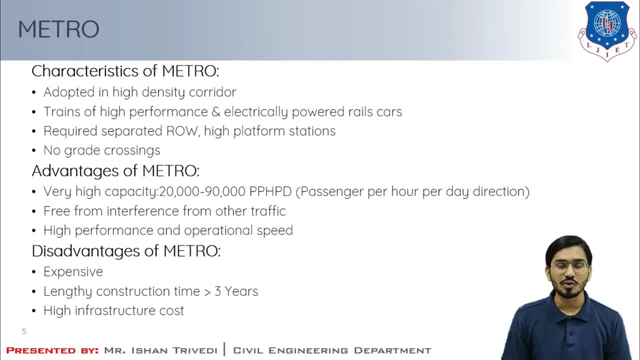 And there is a lengthy construction time, which is almost more than three years Now. if I am talking about the type of metro, These are classified in three parts, that is, subway, heavy rail at grade and elevated Subways are provided where there is highly densified area. 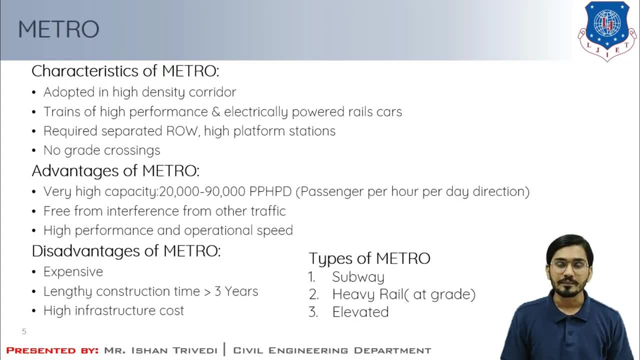 Or you can say highly densely populated area like CBD area In Ahmedabad also. you will find in particularly CBD area in Kalapur. it goes under subway. Here we are eliminating the elevated part and providing access to subway. But what would happen here? Here the cost of construction by constructing this subway is very much high. 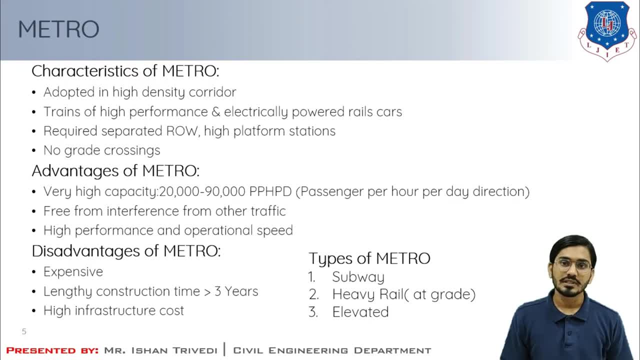 Which is almost four to five times than the construction of rail at grade. Then, if I am talking about heavy rail at grade, In this category particularly, the metro runs over the ballast track, The way our Indian railway runs on the ballast track. 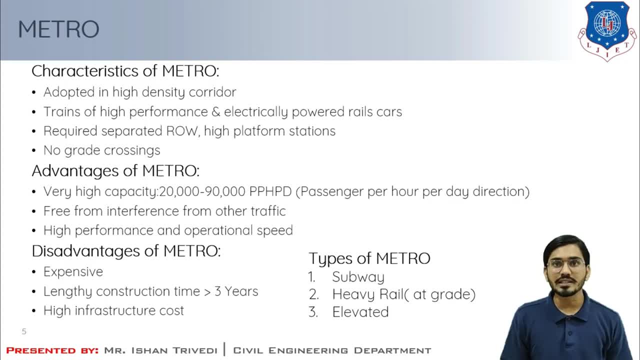 It is one of the cheapest way of flying the metro. Generally, metro at grade stations are provided at the suburban area and the main city. distance Means it connects the suburban area and the main city. Then heavy rail at elevated Instead of operating in the shared right of way the way it has been done in at grade. 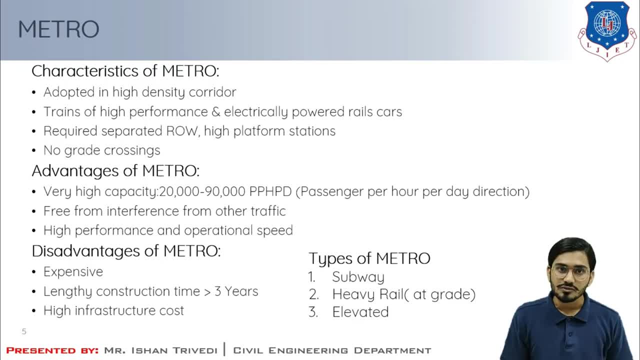 This system is operated on an elevated. It is effective as a metro can be plied with the general traffic. The cost of this construction of elevated metro is twice that of grade. So this is what the introduction of metro. You may have several case studies regarding this metro. 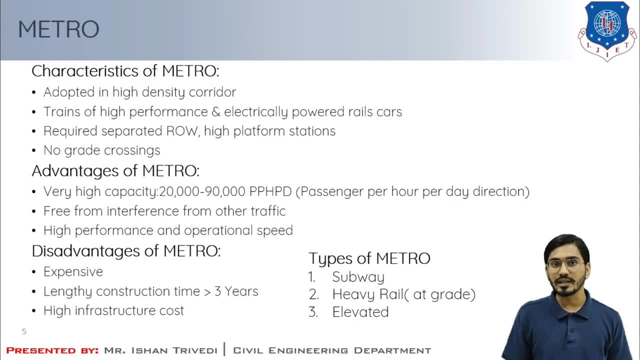 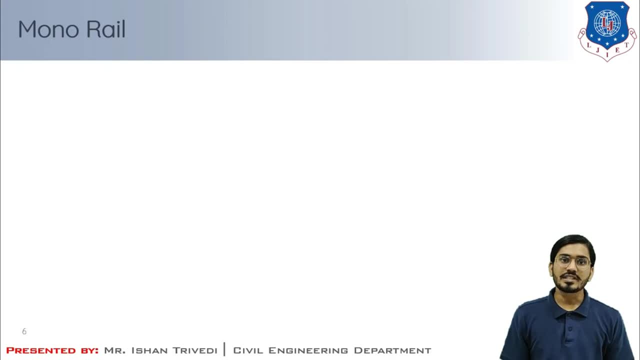 You can refer Delhi metro, Ahmedabad metro as well. Next is monorail system, Means MRS, Which comprise a single rail track With a vehicle suspended from, or you can say straddling, the guided way. Here monorail vehicle are wider than the supporting guided way structure. 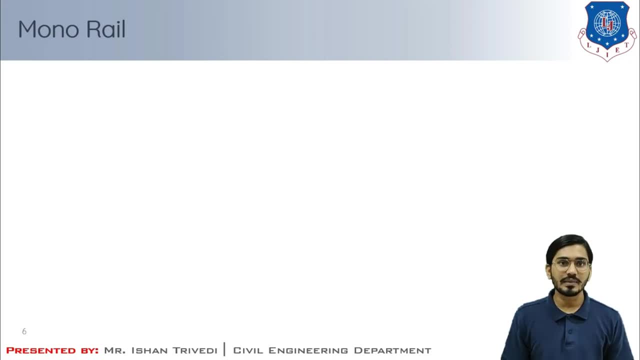 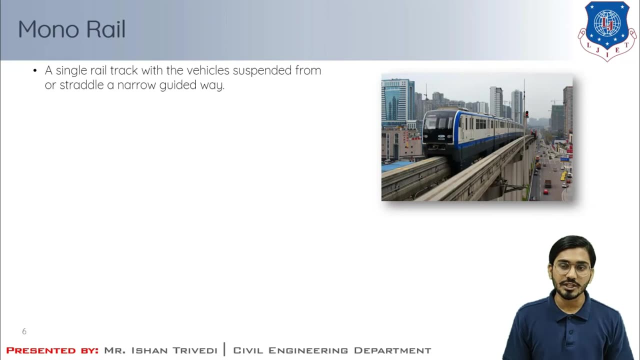 In most of the cases, the rail is elevated, But it can also be at grade or in subway tunnels. Here you can see in this picture Where the guided way is narrower than the platform of the railway, And that's why it requires minimum space in terms of its pillar and gutter as well. 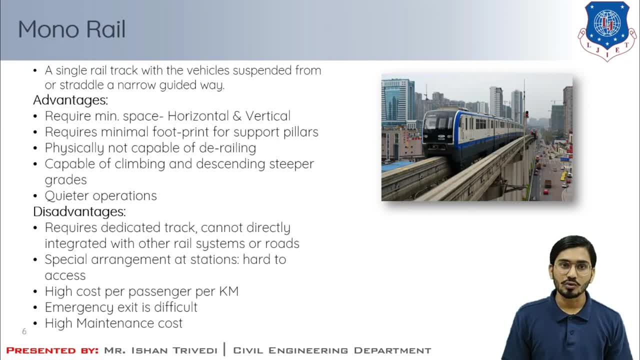 Now the advantages and disadvantages of monorail. As I said, it requires minimum space in horizontally and vertically. It requires minimum space for footprint, For support of pillar. It is physically not capable of derailing And that is one of the major advantage. 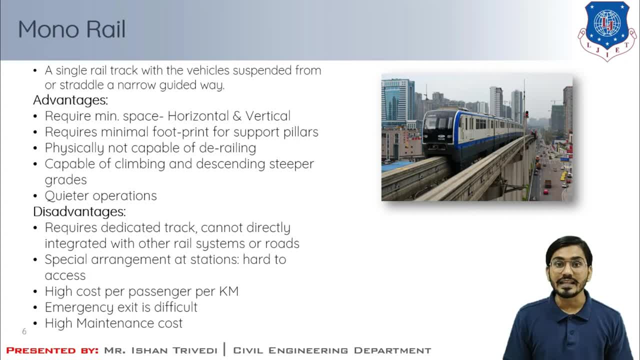 It is capable of climbing and descending the steeper gradient as well And there is quieter operation, are easier Means the turning and changing of the track is easier And it is easy to operate. If I am talking about the disadvantages of monorail, 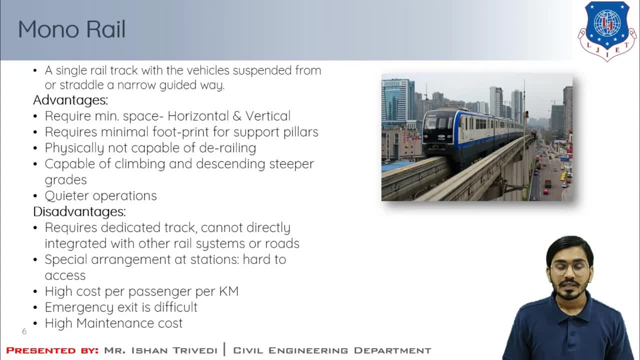 Then it requires a dedicated track And this track cannot be directly integrated with any other type of rail system or route. The stations require special arrangement and which is hard to access. There is higher cost per passenger per kilometer And the emergency exit is very difficult here. 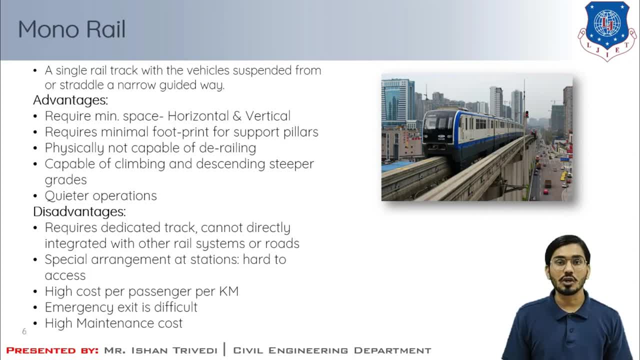 And, at last, the maintenance cost are also higher. If I am talking about the types of monorail, Then there are suspended type, straddle type and maglev monorail. If I am talking about the suspended type monorail, Then in this type a single steel rail is suspended from an elevated structure. 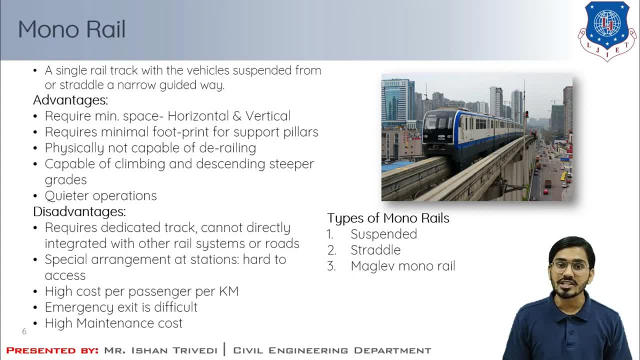 Means. instead of RCC gutter, there is a steel structure And the elevated structure is also of a strip And along with a single rail runs. The vehicle weight is supported by the rails, And this type of rail is mostly used in the amusement park. 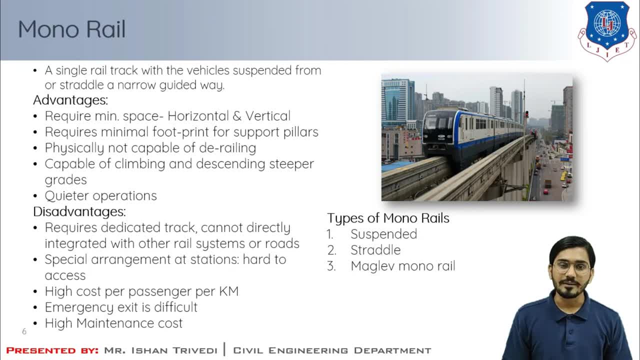 Next is straddle type. In this type the coaches are moved over a RCC beam And supported over RCC column. This type of system is most suitable for the congested areas like CBD. Then next is maglev monorail. Here the maglev monorail operates on the same principle, that is, of a straddle monorail. 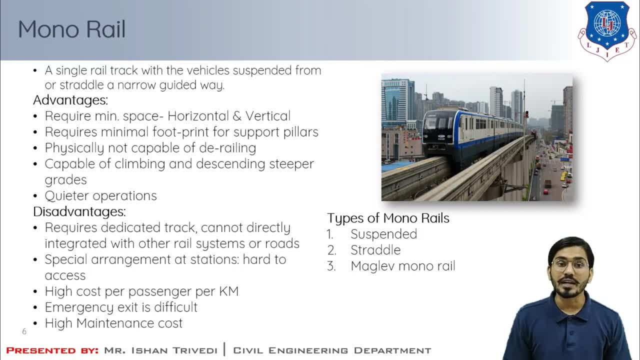 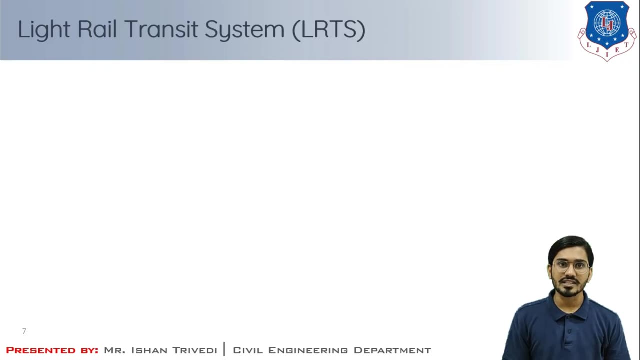 But here the difference is that it operates on a different technology, And that is the magnetic levitation, And it is one of the most faster and energy efficient technology. Next system is light rail transit system, LRTS. These systems are being increasingly developed. 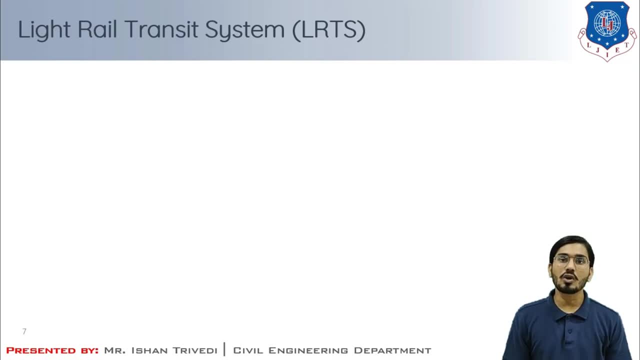 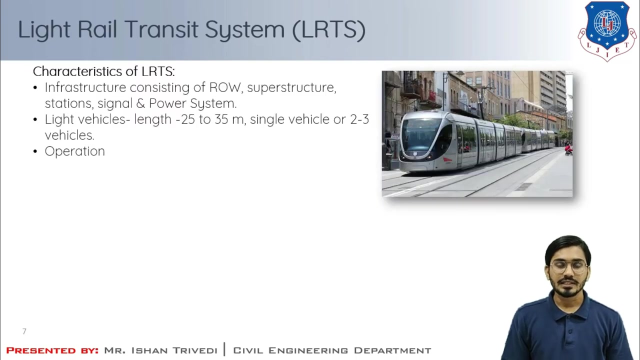 And being increasingly used in the urban areas all over the world As a mode of rail based on public transport. You can say it is one of the modified version of tram Which share the right of way along the road system. You can see here the railway track and the road system. 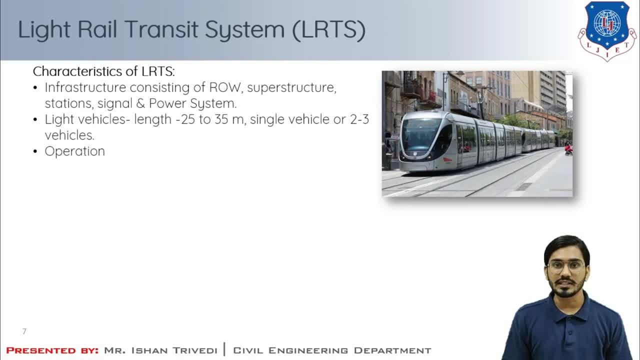 The right of way is being shared among all these two separate type of transit. Here. this LRT uses rail system. LRT uses relatively lighter vehicle and lighter track as well. It can be developed in stages from a modern tramway That shares its right of way with the other traffic. 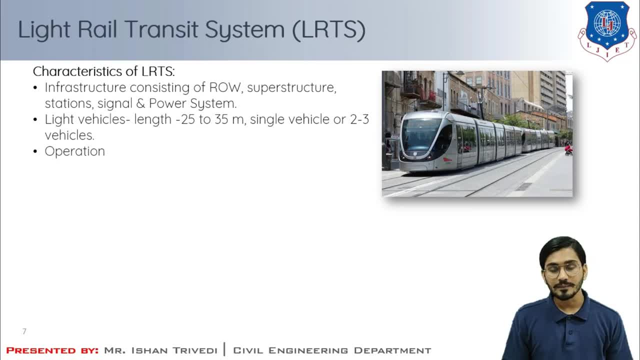 To the rapid transit Means, as I said, that it is one of the modified version. At initial stage, you can provide the tramway And you can just update it based on our requirement And it is one of the modern tramway. So if I am talking about the major components or characteristics of LRT system, 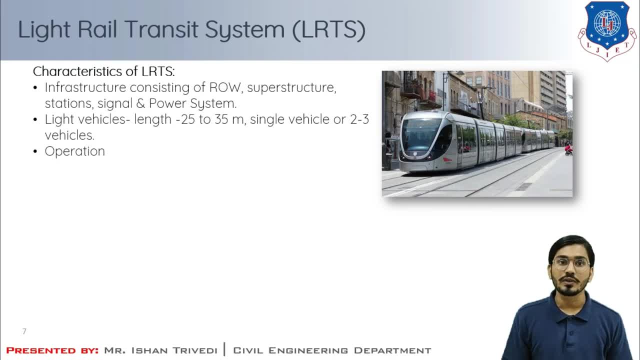 These includes the infrastructure consisting of Right of way, superstructure station, signal and power system as well. These are the light vehicles Which consist of length of 25 meter to 35 meter, Or you can say it is a single vehicle. 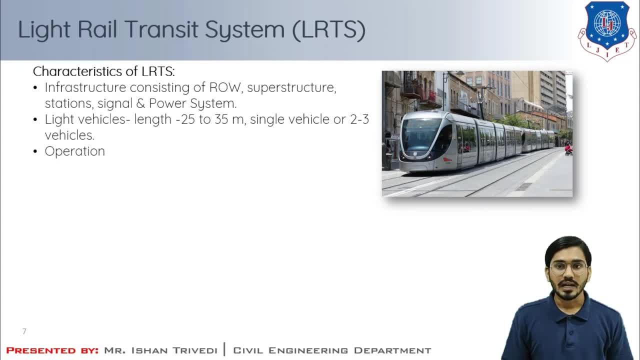 Which is provided with 2 to 3 attached vehicle, Or you can say articulated coaches, And next is the operation. If I am talking about the advantages of LRT, It uses light articulated vehicle, as I said, And its capacity can be higher than the bus system. 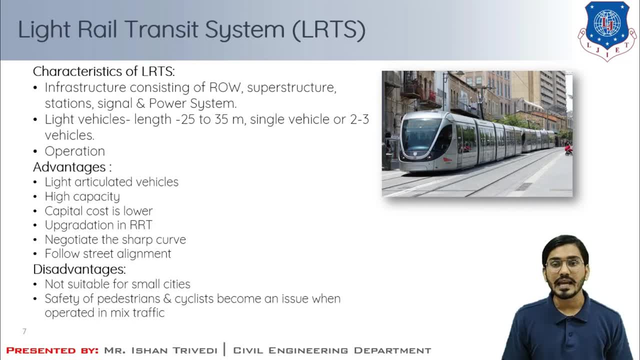 Here the capital cost is lower. That is one of the key benefit of this LRT system. Then it is possible to start as a tram And we can upgrade these rapid rail transit system And their standards As the traffic and the available resources. 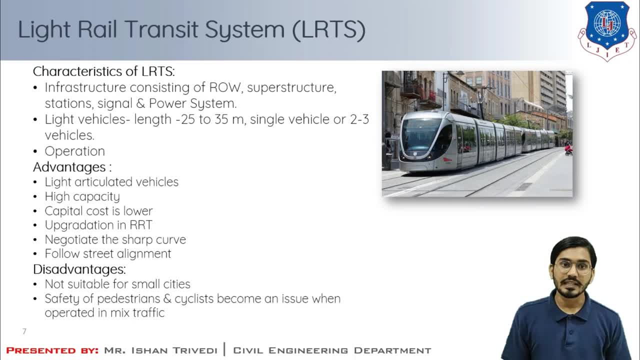 Which increase in the future. It can negotiate the sharp curve about 75 meter radius And it can follow the city street alignment Which is one of the beneficiary part of LRT. If I am talking about the disadvantages of LRT, It is not suitable for the small cities. 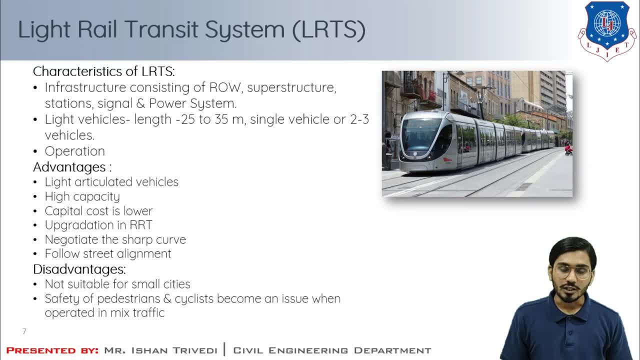 Because of the sharing of the right of way, The safety of pedestrian and the cyclist becomes more important as well. So here we have to take care about pedestrian and the cyclist Which are merging in this mixed traffic conditions, If I am talking about the types of LRT. 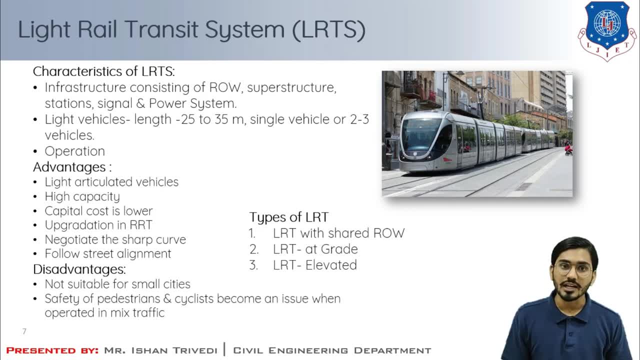 Then these are of LRT with shared right of way, LRT at grade and LRT at elevated. If I am talking about shared right of way LRT system, It is improved version of tram And operated along with the mixed traffic And due to this the speed is significantly low. 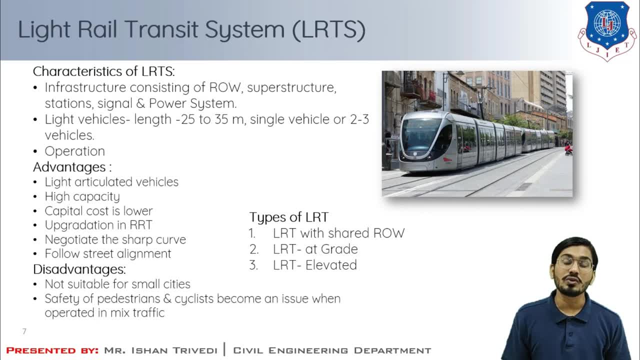 As well as the passenger carrying capacities also reduces. Here the safety becomes the main issue, As it is operated along with the mixed traffic, Then LRT at grade. They are operated at grade with the standard gauge track And the efficiency is significantly more. 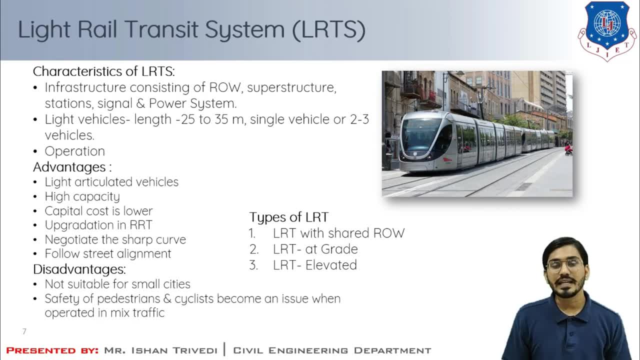 When it compared with the LRT operation in shared right of way, Then LRT at elevated. Instead of operating in the shared right of way, The system is operated in the elevated bridges And it is effective Where the sufficient ROW is near or you can say not available.